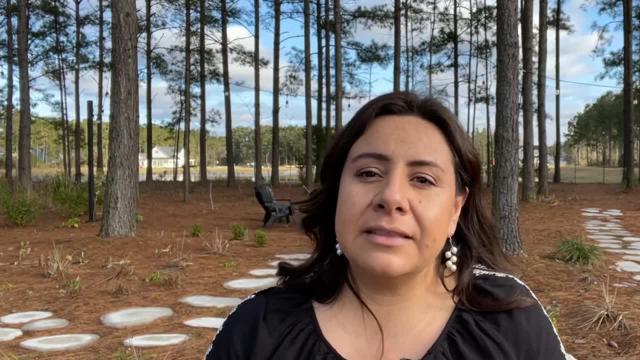 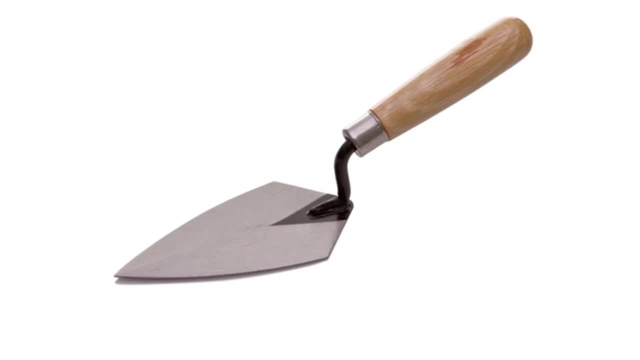 easy to carry around. If you want one, I'm going to share the link in the description and I'll probably make another video so that you know I can tell you all about that. You're also going to need a trowel, okay, something that you can smooth out your stepping stones- The cool thing about 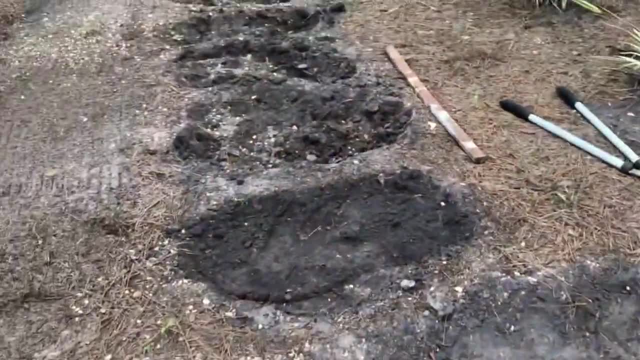 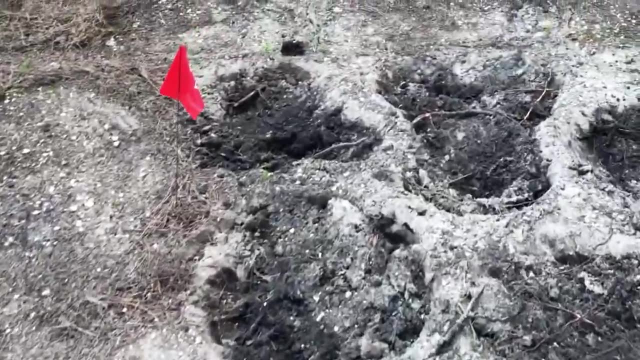 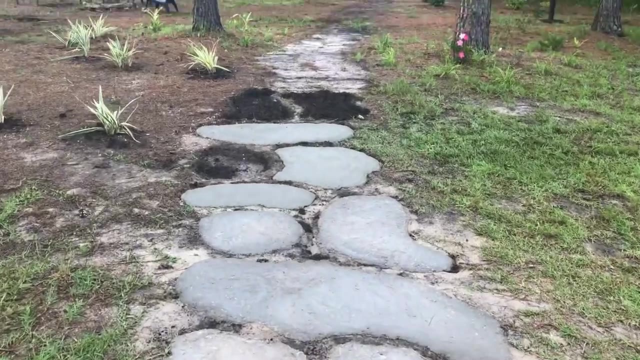 this method is that you don't need a mold. You're going to mark where your stone is going to go right on the ground. That's why you need your marking tool. And also, you're not going to need any pea gravel or any prep work underneath the concrete, because it is going to align right on. 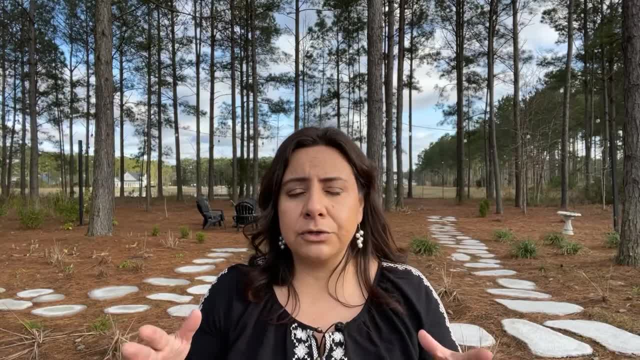 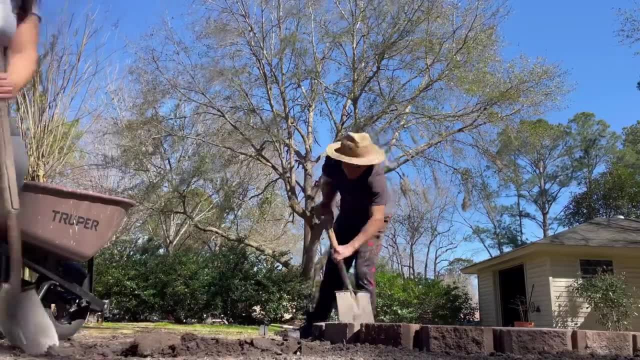 the ground perfectly. You're. basically. what you're going to do is you carve out your mold and then you dig out the dirt around it, So you use that as your perimeter. then you dig the dirt inside and then you leave two inches of depth and then you make sure that it is level, because 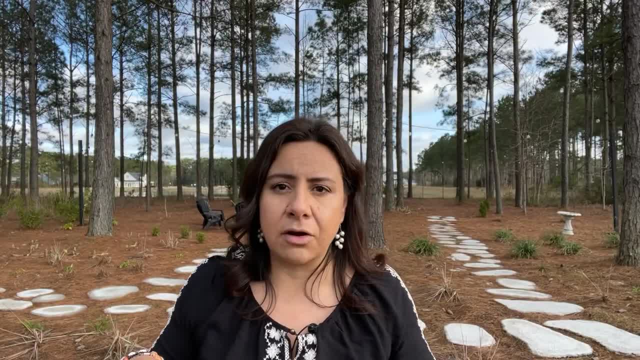 that's a good enough thickness that it's going to fit right on the ground, And then you're going to make sure that it's level, because that's a good enough thickness that it's going to fit right on the ground. Anything heavy can stand on it. We've had our riding mower go through them and they have no. 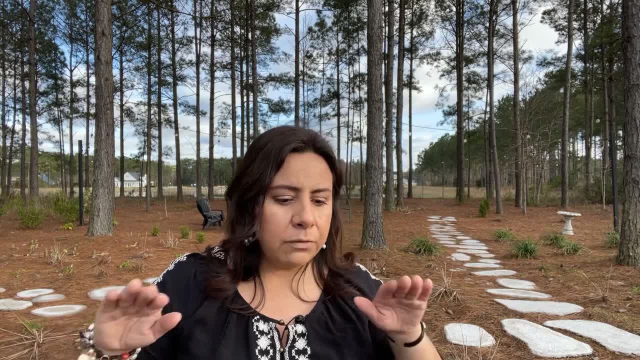 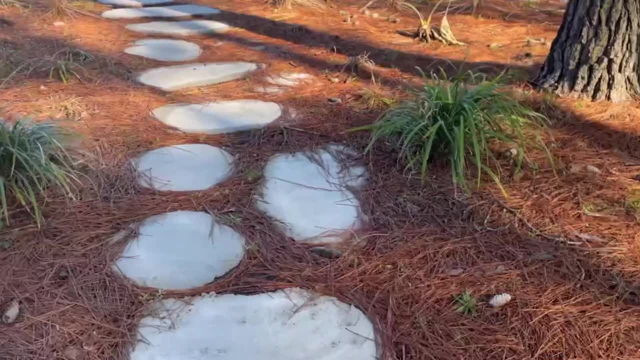 problem. You can decide whether you want them flush to the ground or if you want them a little bit out, if you want them a little bit round, if you want them jagged edges- you can decide exactly how you want them. I ended up making about 75 stones. I feel like I earned the title. 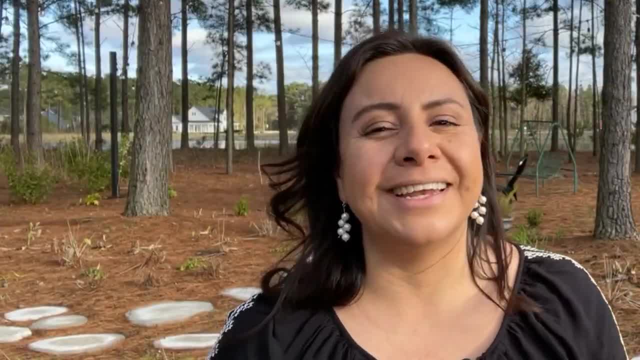 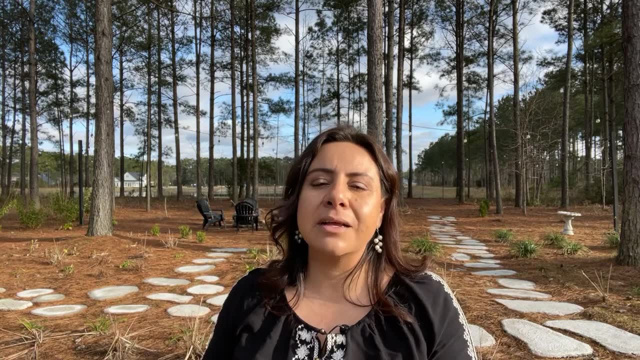 of a stepping stone maker expert, Just kidding. I think this is a really a two-person project. So get your spouse, get your friend, your kids, somebody to help you, because the concrete bags are heavy, So be careful with your back, and it actually can. 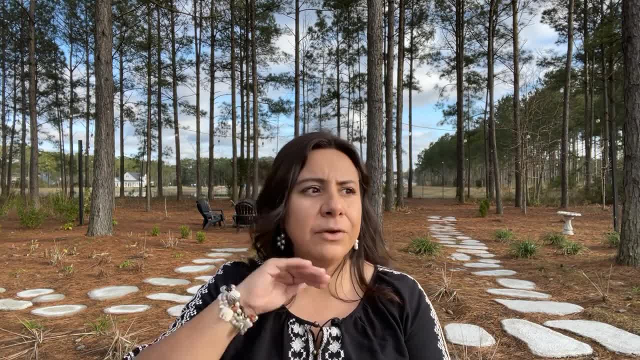 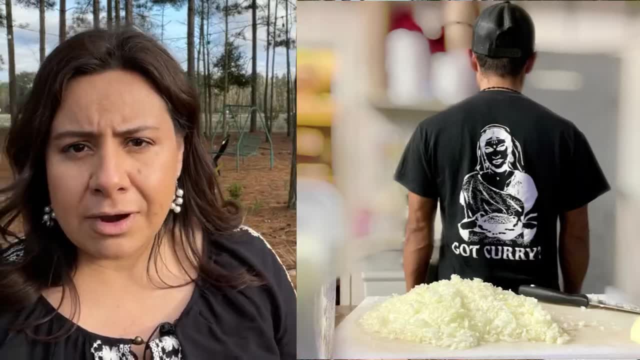 dry pretty fast, So if you're working alone, you might have to go get something, or you need more concrete. I have a family member that helped me with this project, and he works at a restaurant, and so we would create stones in the morning before he went to work. 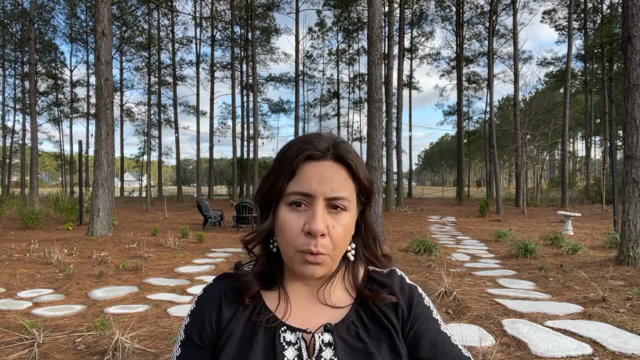 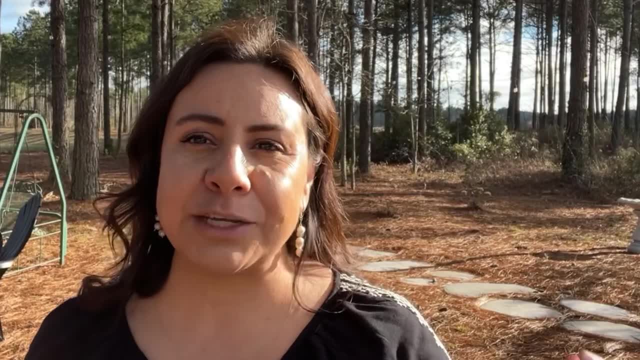 You need to be able to move quickly, and so one person pouring while the other person is spreading and smoothing and kind of shaping the stone is perfect. If you have some questions, make sure you comment them below, as I do read them and I will respond. 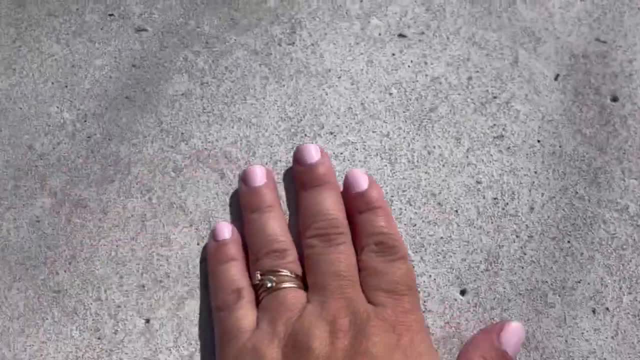 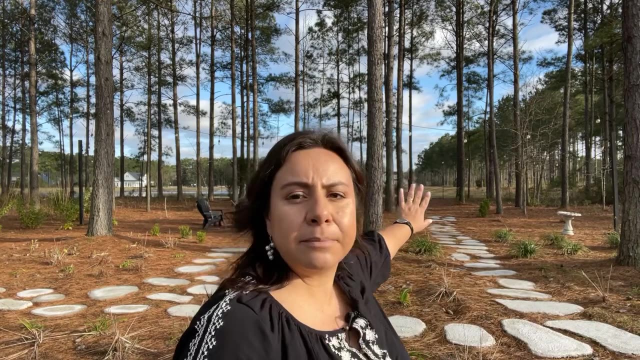 The ending stepping stones are much better than the beginning ones. You know they were smoother, they were just prettier. So here's some tips. Start from the back- So that's the back of my area- At the most inconspicuous places. first, Pick a day to do this when it's not raining. 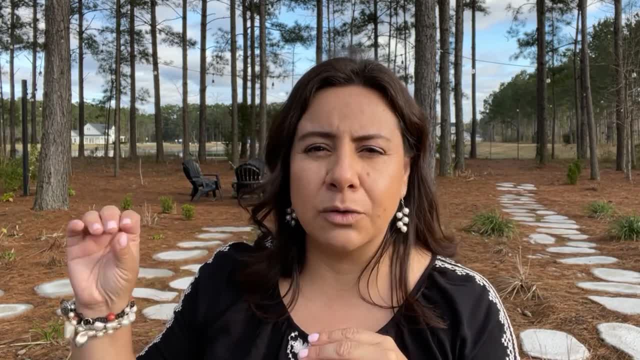 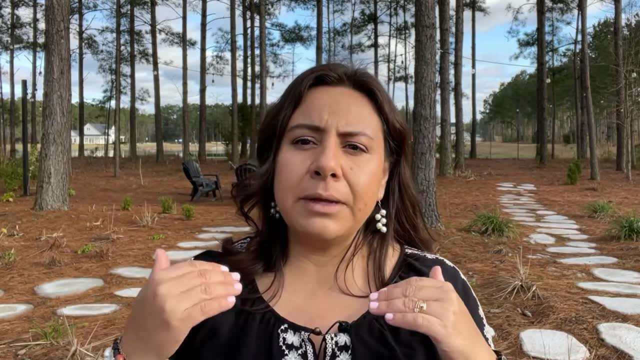 because the rain tends to like do something to the back of the stone. So if you're going to do this to the concrete where it leaves little marks, if it's going to rain maybe later in the day, wait at least six hours so it doesn't get any rain. But ideally it would be a not rainy day. 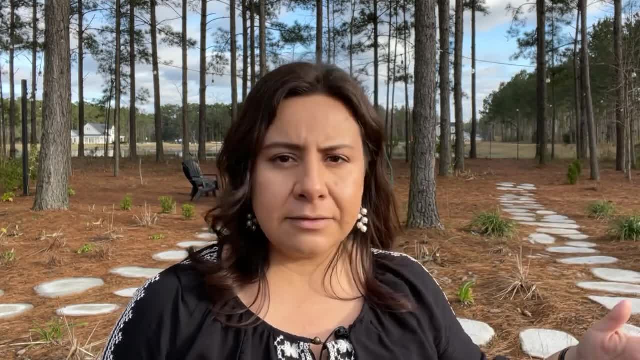 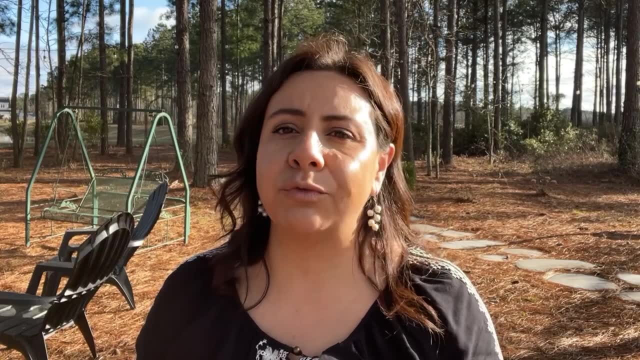 where it has a whole day to cure and then the next day it could get rain And actually that's not even bad. It actually helps it to set even more. I would have liked a more organic, natural feel And, even though I'm happy with how they turned out, I would have liked to add some colors. 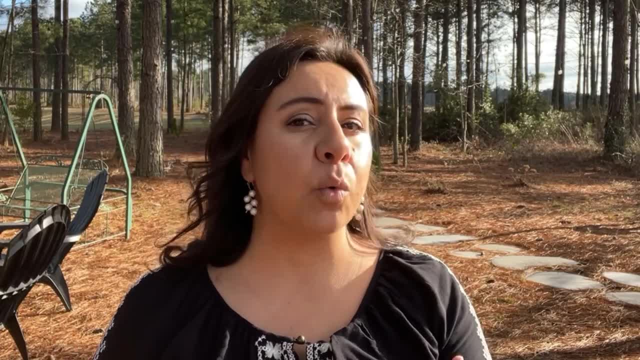 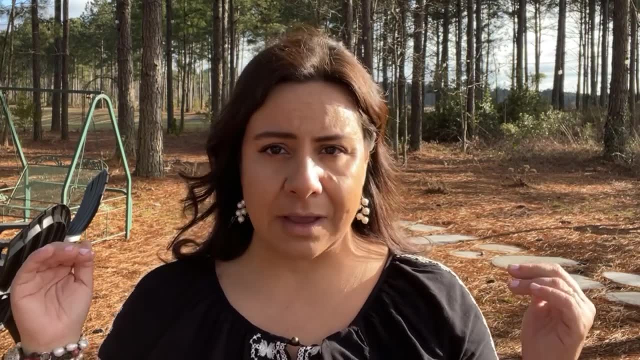 The other thing I want you to know is not to step on them for at least I'd say a week, because we did crack one, that we stepped on on it too soon. So just be cautious. One, two weeks is ideal. I was 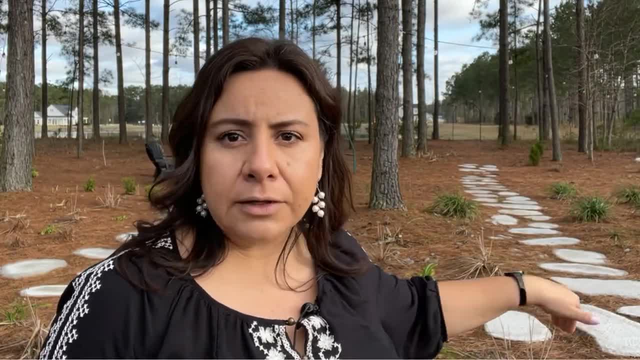 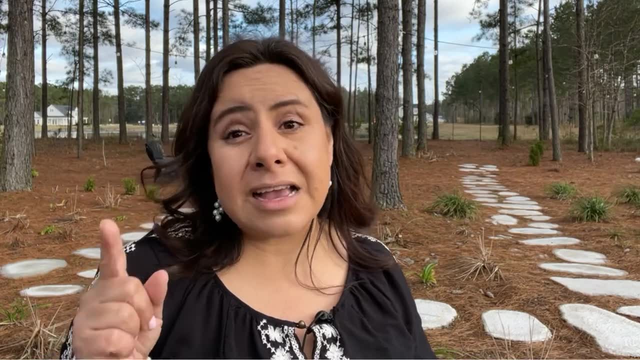 afraid that when I went ahead and did this on directly on the ground, that I would be forced to have it stay there forever. That's not true. You can actually move this, And I actually did change my mind about the location of some of these stepping stones. You need to be able to let it cure. 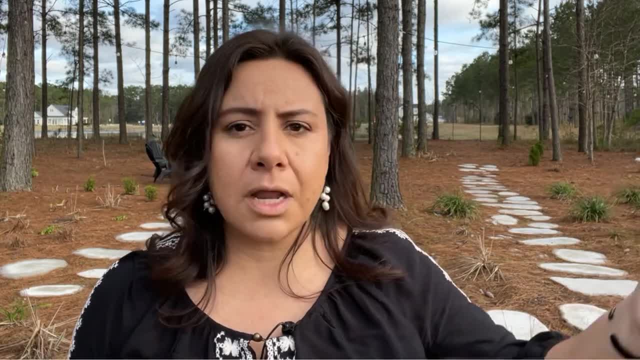 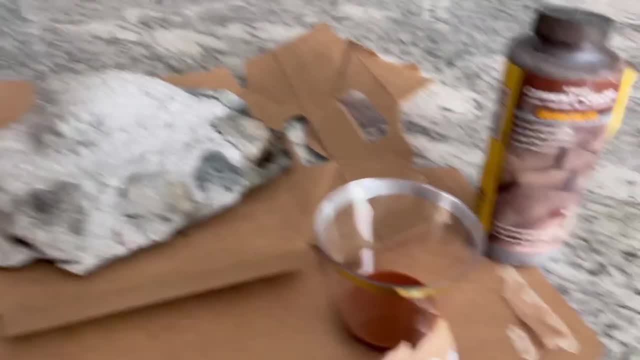 enough that it doesn't crack on you And you could just use it in another part of your garden. But they are removable, So I'm going to use my little brush. I've poured this concrete cement color by Quikrete And this: 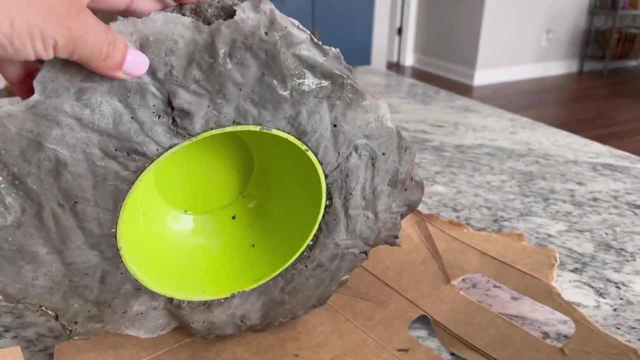 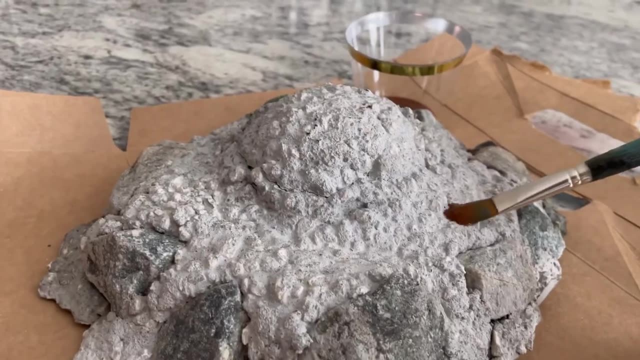 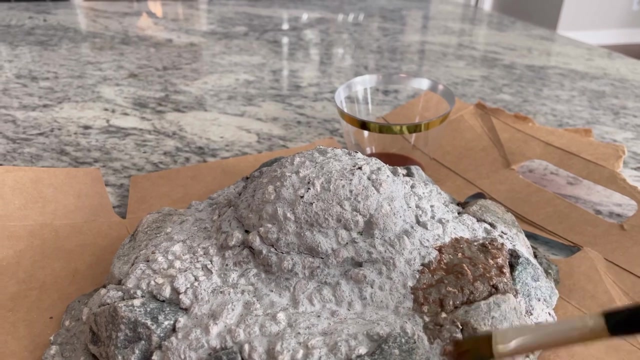 is the color brown. I kind of made it hollowed in here because I use it to cover an extension cord that goes out to the back. So let's try this out and see if it works. I have no clue if this is going to work, because this is after the fact, So I don't know if this will even do anything to it. 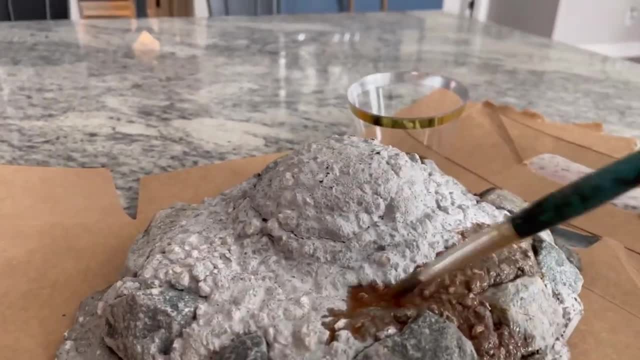 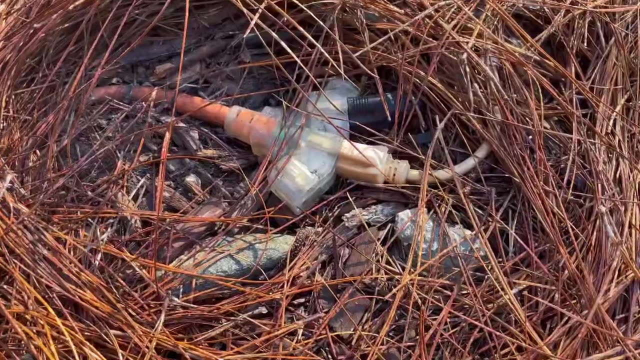 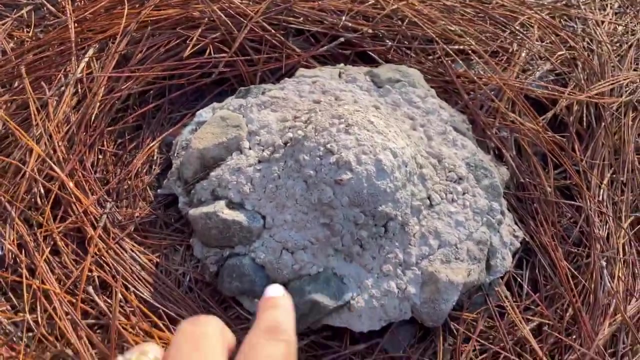 This thing smells disgusting, I have to tell you. Here we are, where I typically cover this. That's what I use it for in another part of my garden, And this is what the stone looks like after it's had a little bit of color. You can see.